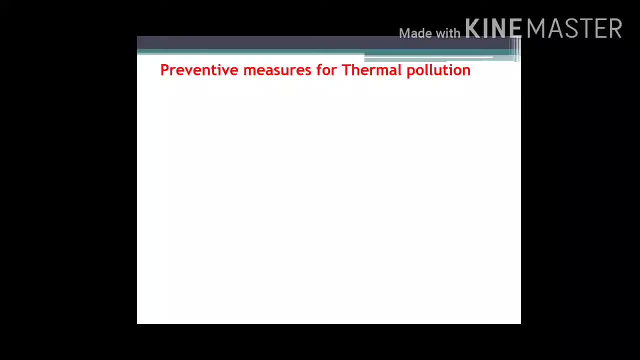 which temperature of the water rises and how this can be prevented. Now, the first way is use of cooling towers and artificial leaks. Actually, in the industries, water is used as a coolant and the hot water generated in the industries when discharged into the water bodies. as such, it can raise the average temperature of the water and can make the 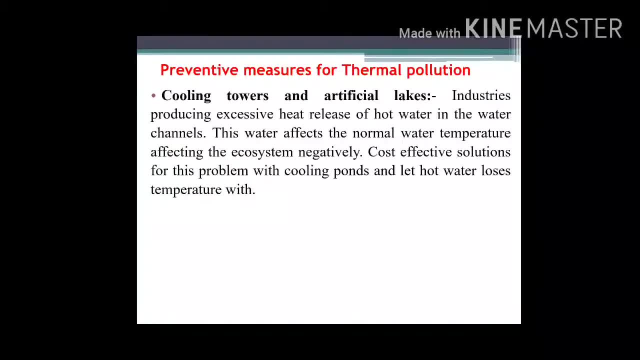 unfit for living of aquatic organisms. Now we should use cooling towers and artificial leaks for the temporary storage of the hot water so that the temperature of the water lower down, and after some time we should discard that water into the main water bodies. Now next is save electricity. 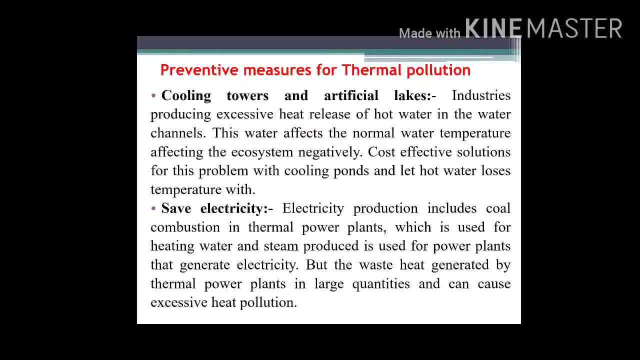 As we know that electricity is produced by thermal power plants in which coal is burned, nuclear power plants. These all power plants make the water hot and when that hot water is discharged into the water bodies can cause thermal pollution. So we should save electricity so that there will be need of generation of less electricity. 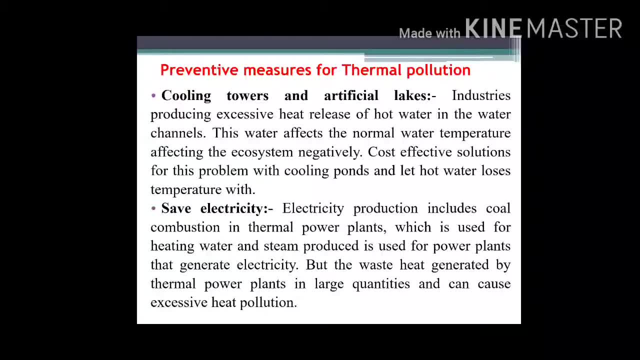 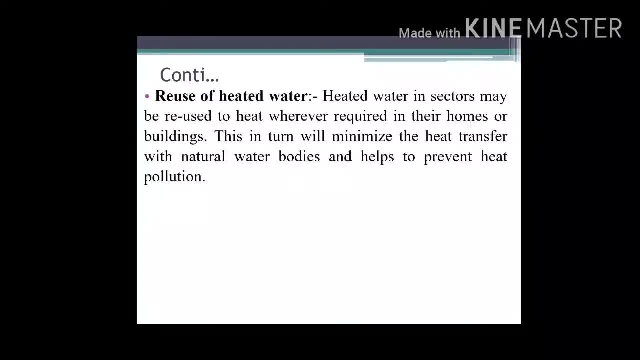 and will reduce the thermal pollution. Now, next is reuse of heated water, As we know that in industries and different commercial activities which generate hot water, that hot water can be used wherever required: in the homes, in the buildings, wherever hot water is required. 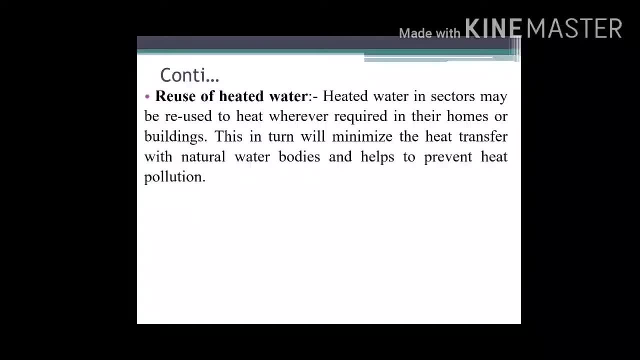 hot water can be used there, and when the water becomes of, becomes at low temperature, then it should be released into the main water bodies. it should also prevent the thermal pollution of water now. next is environmental awareness. all should be aware about the environment or the negative consequences of the pollution of the environment, and that can also prevent the 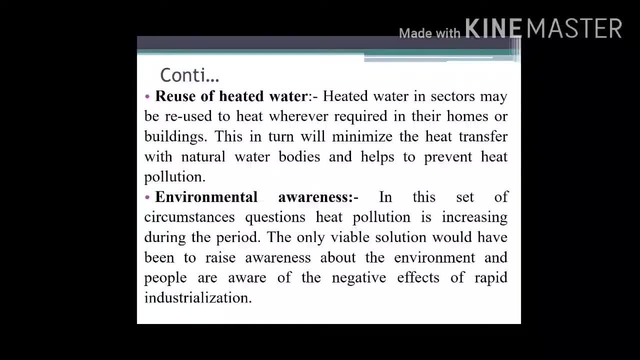 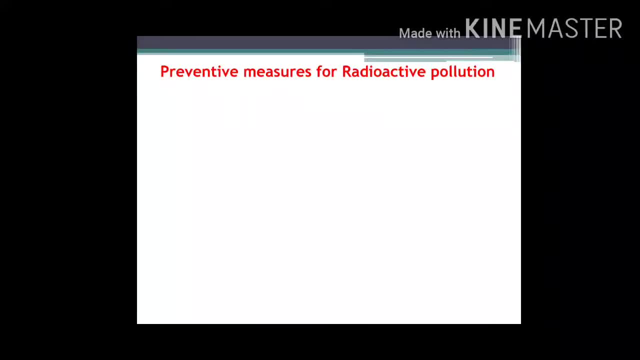 water pollution or the thermal pollution of the water. now next is preventive measures for radioactive pollution. radioactive elements should be stored in a proper way. there should be a used specific kind of con kinds of containers so that leakage could not occur, because their leakage can can emit hazardous radiations into the environment, and so radioactive elements should be stored. 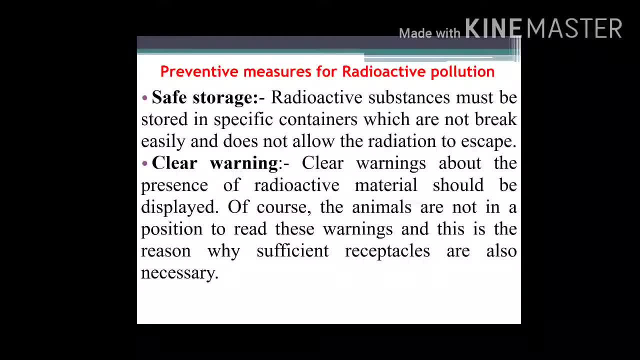 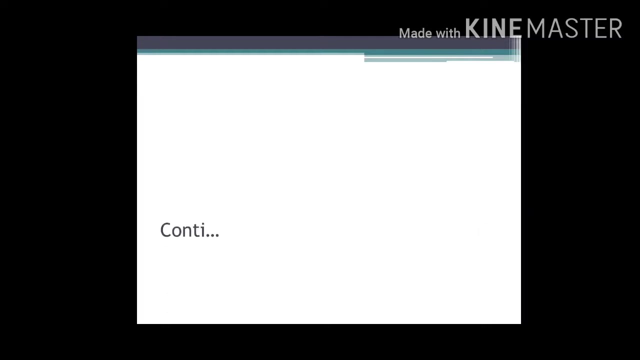 safely clear warnings. clear warnings should be displayed on the reasons where radioactive materials have been kept, as you all know that animals cannot read these warnings, so we should use sufficient receptacles so that animals could not reach to the site where radioactive elements have been stored. now next is alternate sources of energy. we should search for alternate sources of energy. 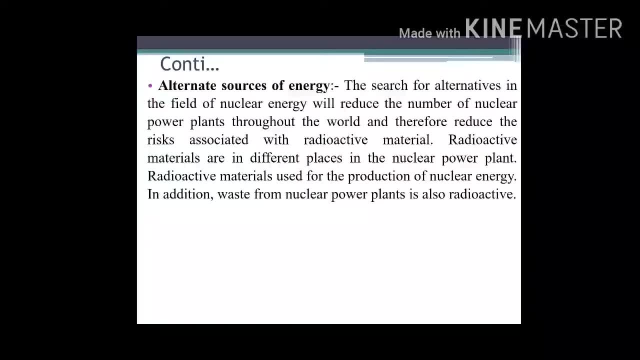 so we will have different sources of energy. written short term at the end of the articlea: sources of energy. we should not use nuclear power plants for the generation of electricity because in the nuclear power plants radioactive elements are used and there is a risk of leakage of these radioactive elements from the nuclear power plants and it can cause the radioactive 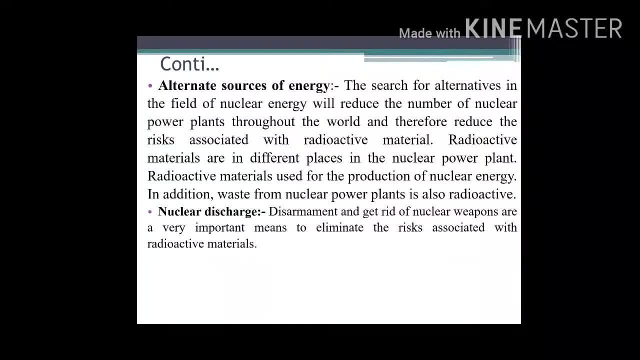 pollution. next is nuclear discharge. that means nuclear weapons are a very important means to eliminate the risk associated with radioactive materials. so we we should get rid of nuclear weapons because these can these can produce the radioactive materials into the environment and that can produce hazardous radiations. now next is proper disposal. 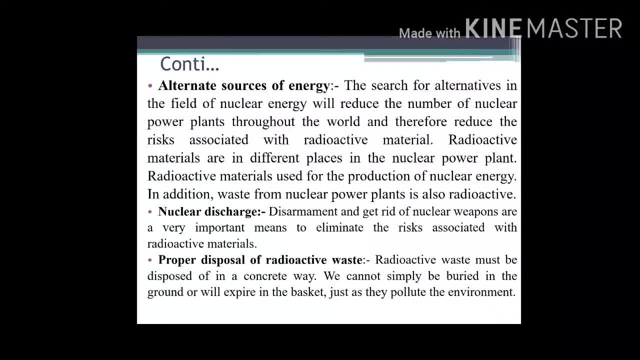 of radioactive waste. radioactive waste may emit hazardous radiation, so it should be disposed in a concrete way. it should be disposed. it should not be buried in the ground because it can cause soil pollution. it should be. it should not kept in the containers which can leak you. okay. so these should be disposed properly so that they could not contaminate the environment. 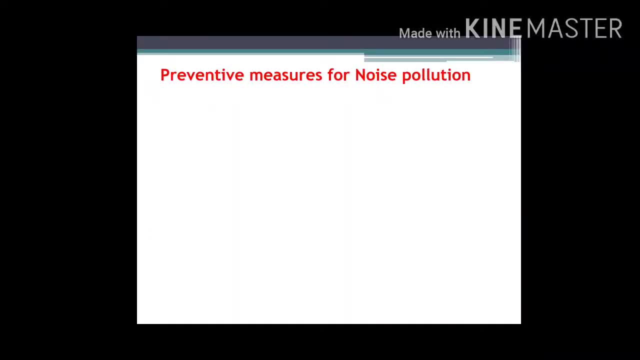 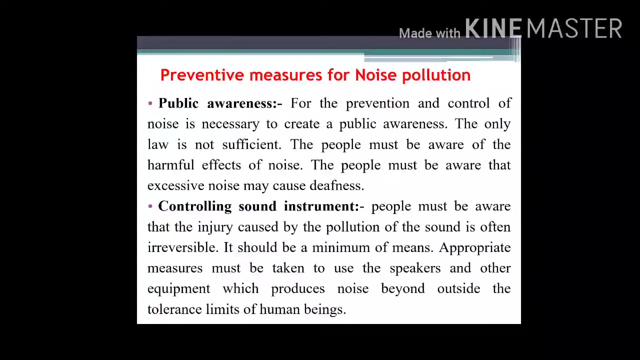 now. next are the preventive measures for noise pollution. first one is public awareness. public should be aware about the control of noise, because excessive noise can produce health effects like deafness. next is controlling sound instruments. people should not use speakers and other sound excessive sound producing equipments, because these excessive sound producing equipments can. 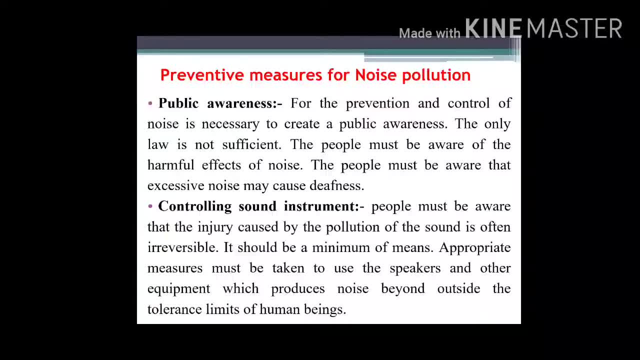 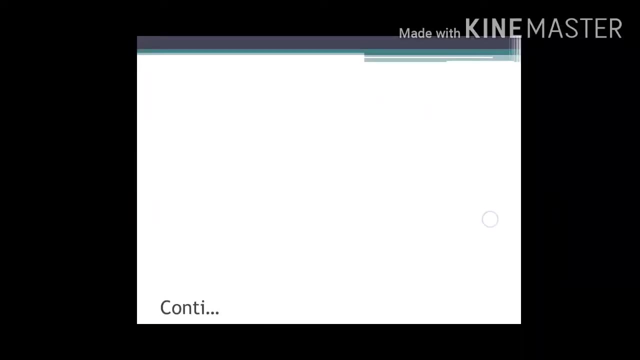 cause. noise pollution can cause hazardous effects on the human beings because there is a limit of said. it is a type of noise Germans are wired into theилось to produce noise which would damage the sounds of these systems. but they may create тут like a sound can make your ears. 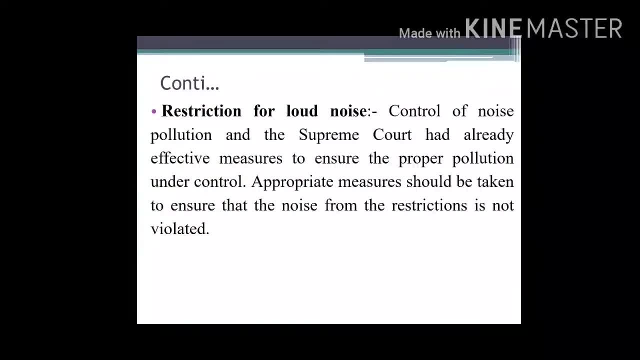 pinch uup, aand, etc. and therefore we we welcome the كلام by, for the human in this lass and the sound beyond that limit can cause the damage to the ear of the human beings. now the next is restriction for loud noise. the, Im feel, is the distinction. for loud noise there should be laws. they should be laws for the control anna noise pollution appellepiece. there should be laws for the control of noise pollution appropriately. 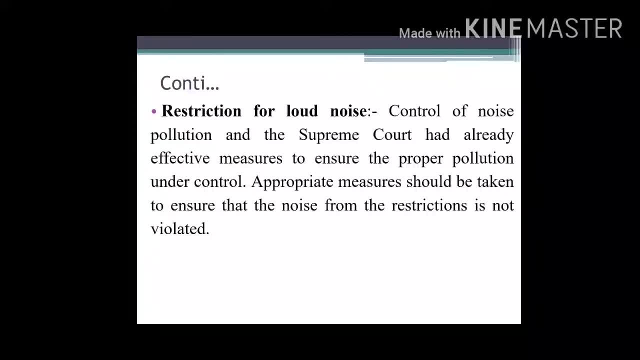 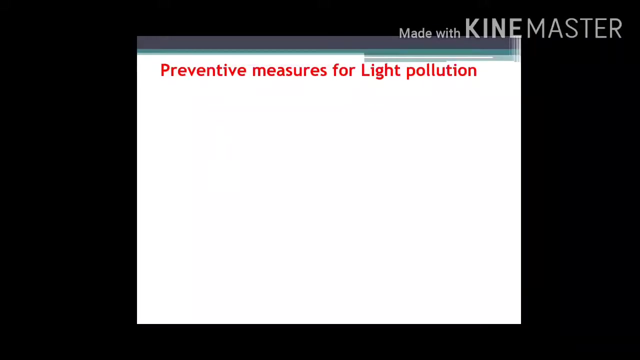 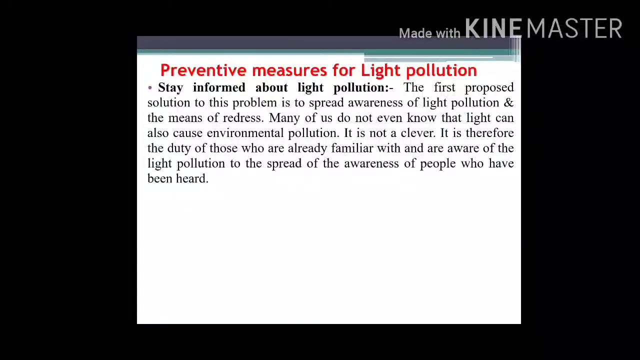 control of noise pollution. Appropriate measures should be taken to ensure that noise from the restrictions is not violated. Firecrackers should be banned or should be avoided, because these also cause noise pollution. Now next are preventive measures for light pollution. First one is: stay informed about the light pollution. Light pollution also.